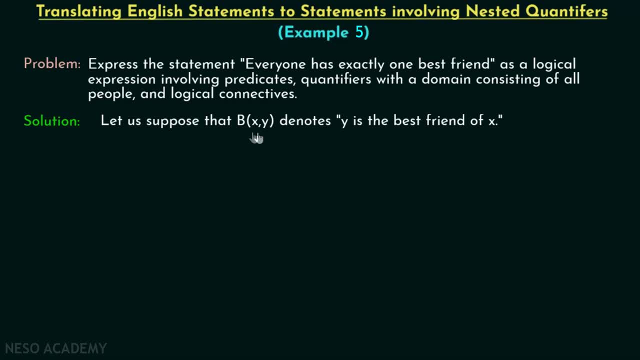 y is the best friend of x. This is a propositional function which denotes this statement. Now, the statement is: everyone has exactly one best friend. We can write this: as for all x, x has exactly one best friend, Isn't that so? 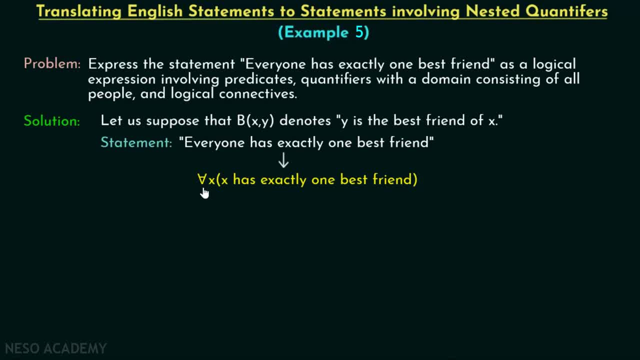 Here we are representing everyone by for all quantifier, because we are talking about everyone, right? Everyone has exactly one best friend means for all x. x has exactly one best friend. Now can we say that for all x there exist, y, bx comma y is actually equivalent to for all x. 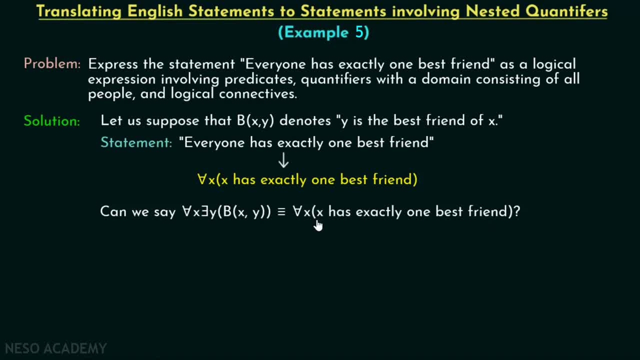 x has exactly one best friend. Can we just replace this x has exactly one best friend by there exist y, bx comma y? No right, Because for all x there exist y, bx comma y says for every x there exist some y, such that y is the best friend of x. There could be more than one. 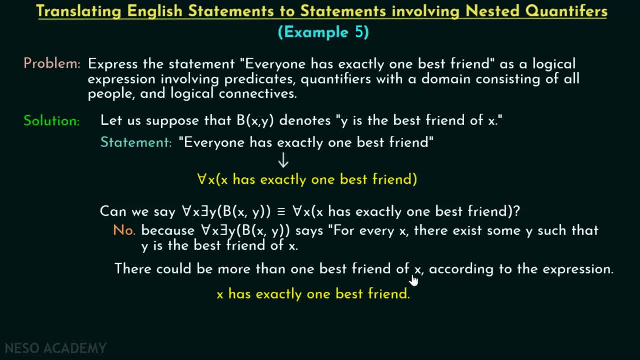 best friend of x. right, It might be possible that there would be more than one best friends of x. Now, if we say that for all x, there exist y, bx, comma y, it might be possible that there could be more than one best friends of x. But according to the question, we have to represent everyone. 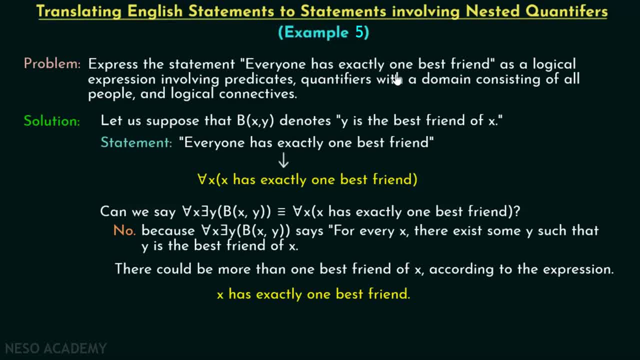 has exactly one best friend. Exactly one, not at least one There exist. y is actually representing at least one, Okay. So there is a difference between exactly one and at least one, Okay. According to the expression, x has exactly one best friend. So we cannot say that for all x, there exist y. 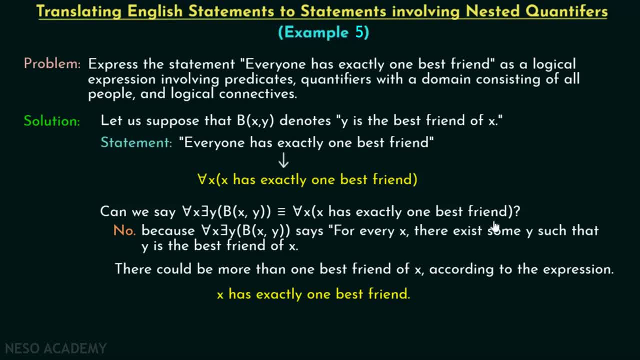 bx comma. y is equivalent to for all x. x has exactly one best friend. Okay, Now suppose that y is the best friend and there is no person in the world other than y who is the best friend of x. If you want to represent exactly one best friend, then we have to do something like this. We can. 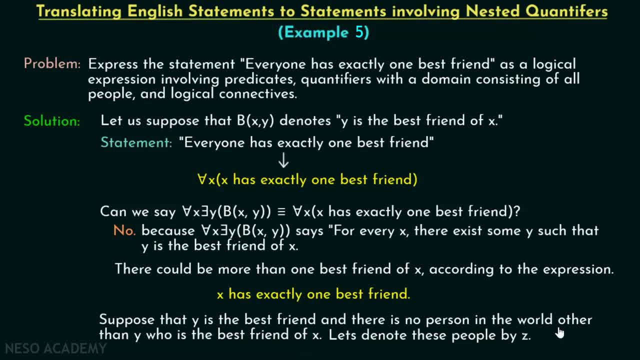 let that y is the best friend of x And there is no person in the world other than y who is the best friend of x. Then only we can say that everyone has exactly one best friend. Let's denote these people by z, Let's say everyone apart. 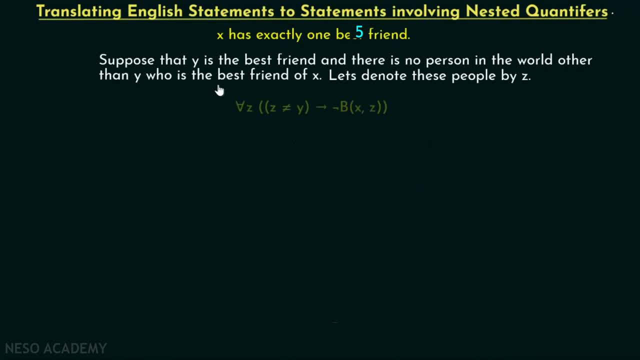 from y are represented by z. Okay, Now the expression could be for all z. z not equal to y implies not bx comma z Here. this represents all people in this world. Right? This represents other than y: All people in this world.